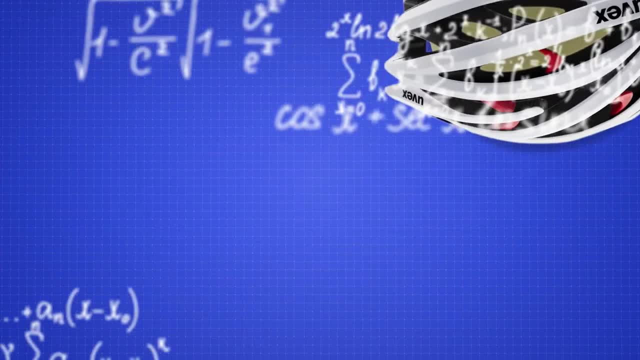 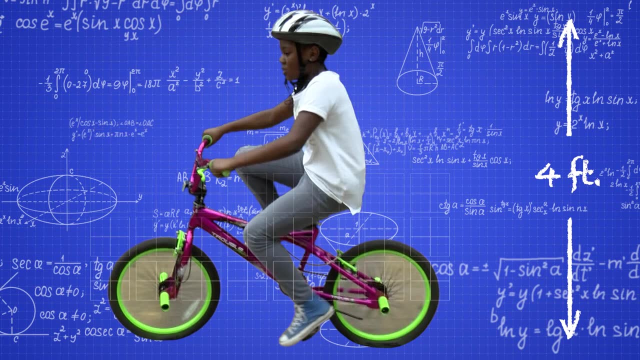 to stand in for your melon. Here comes the science. Come here science. I'm trapped. GO, GO, GO, GO. when you ride a bike, your head is about four feet from the ground. when your head falls from that height, look at what happens, just like an unprotected cell. 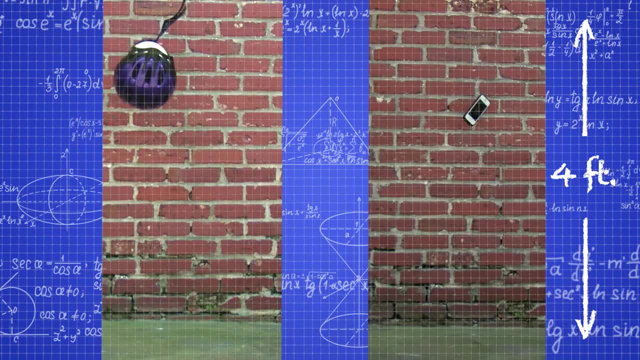 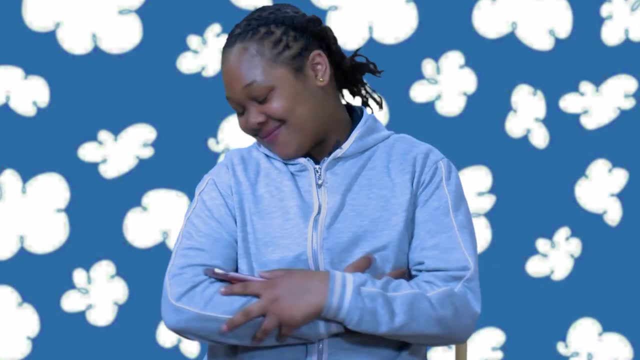 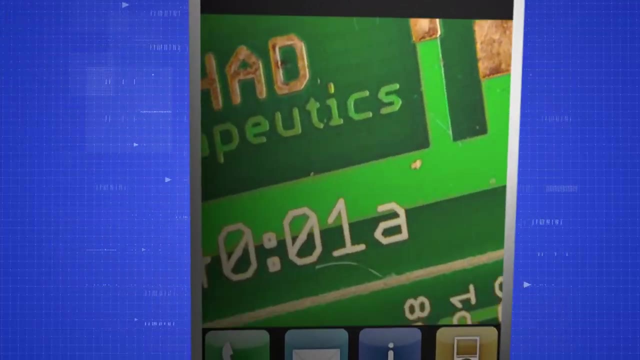 phone, cell phone cases and bike helmets work the same way. they take the impact. so your phone and your brain don't have to so watch your cell phone better than your brain. your brain is a lot like a cell phone. the computer chips, processors and other electronics inside your cell phone allow it to do all the 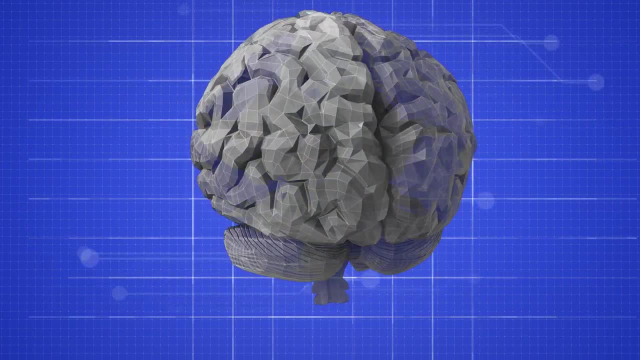 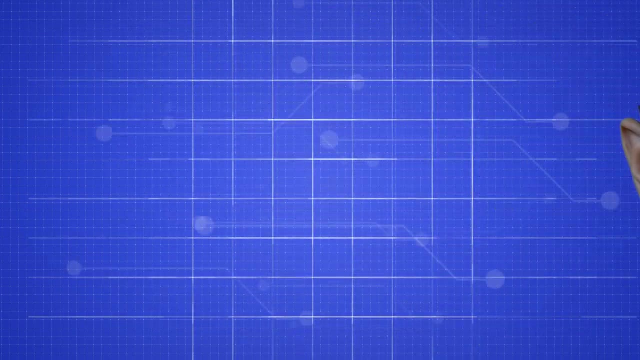 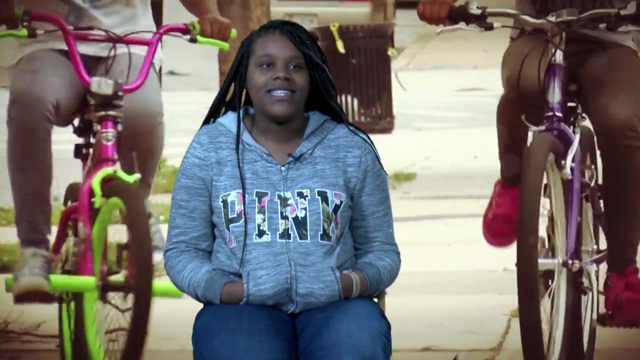 things it does. just like your brain allows you and your body to do all the things you do like. see here, remember things: walk and talk. and just like a cell phone. when your brain gets damaged, it might not work the same way. after a brain injury, you won't be the same. you're just like you don't talk- the same. 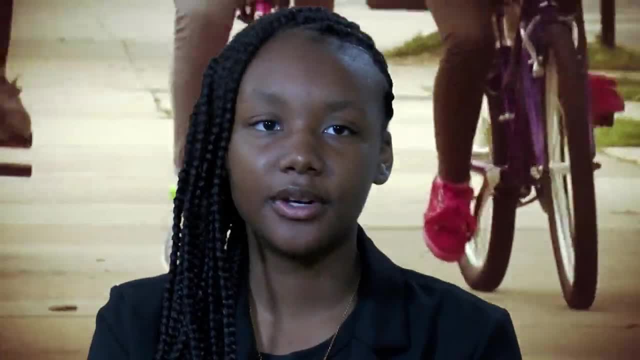 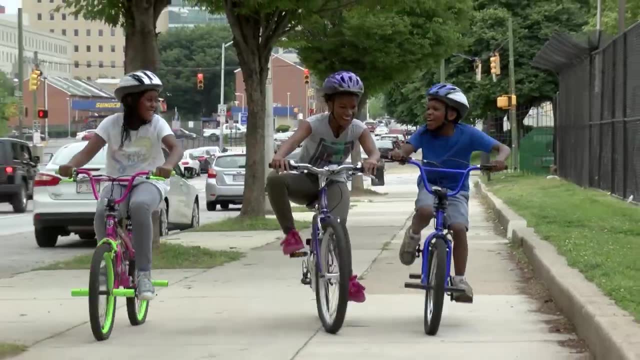 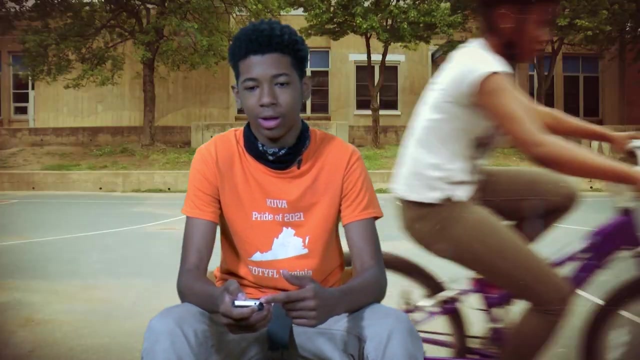 or walk the same. you only have one brain, who you're gonna get a ring from. it's not like you can go buy a new brain, so you make the call. if you've got a phone, you need a case. if you've got a head, you need a helmet. if you're on a bike with no helmet and if you fall, that 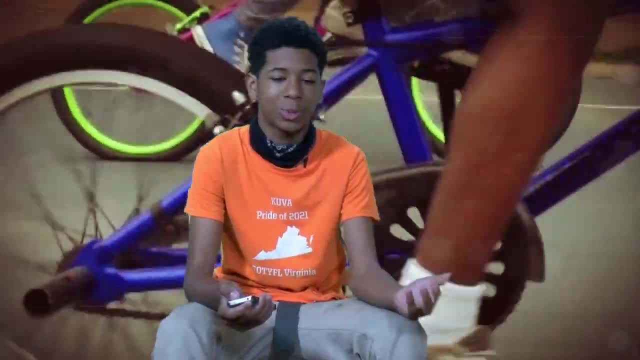 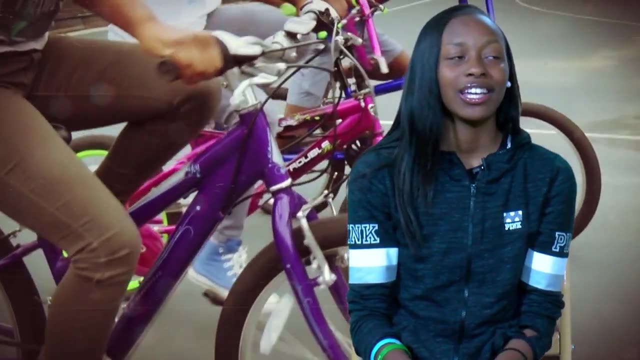 can actually crack your skull, you will go to the hospital, you might have to get stitches and just be a whole lot of drama if you wear your helmet, like you're now aware of what can actually happen, because when I'm riding a bike I'll be more careful when I wear a helmet, because I know 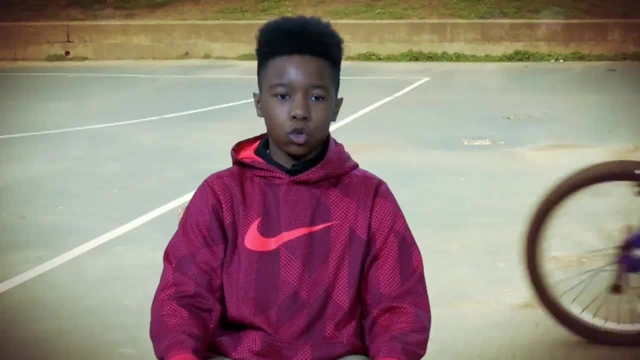 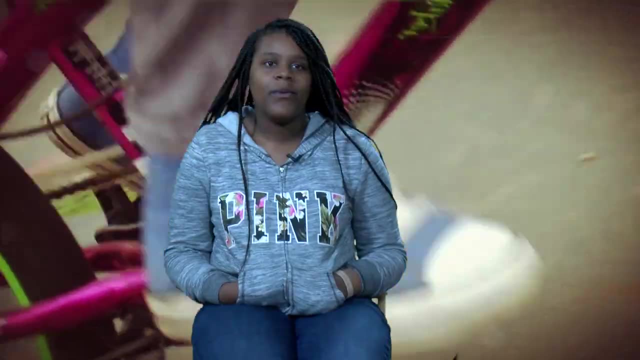 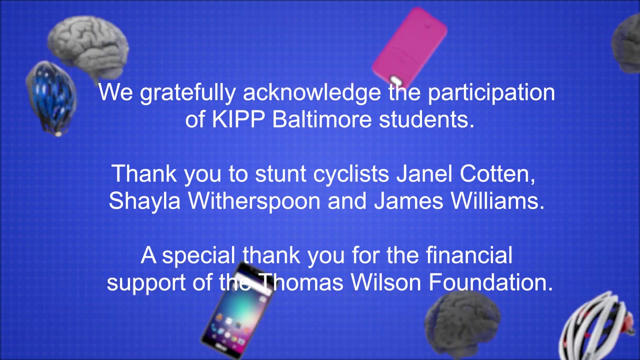 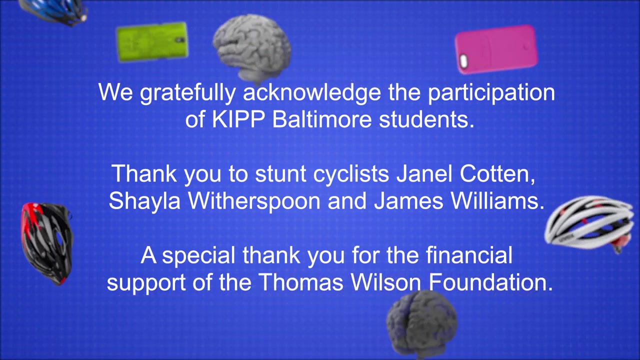 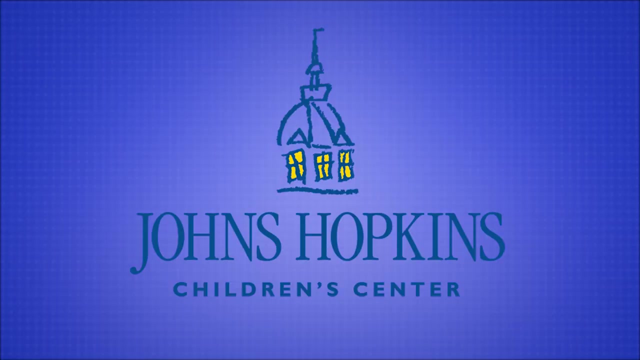 the consequences of not wearing a helmet. you make the call. will you wear a bike helmet every time you ride? you make the call. will you wear a bike helmet every time you ride? you make the call. will you wear a bike helmet every time? you don't wear your helmet every time you. 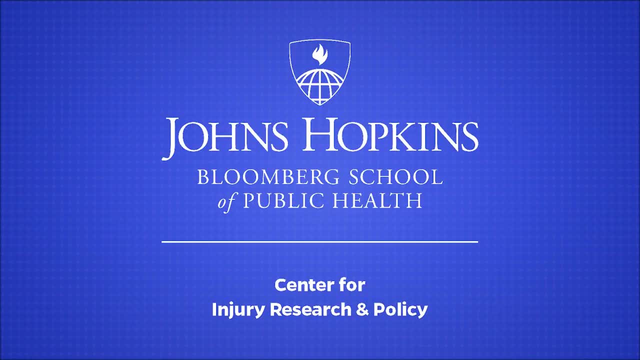 get hit by a bike if you don't wear a helmet. you make things harder. you want to sign to know something. sometimes some schools are like, hey, we want to make sure that way they don't say it every time. just think like that when you get to. hospital, don't think like without real teacher.